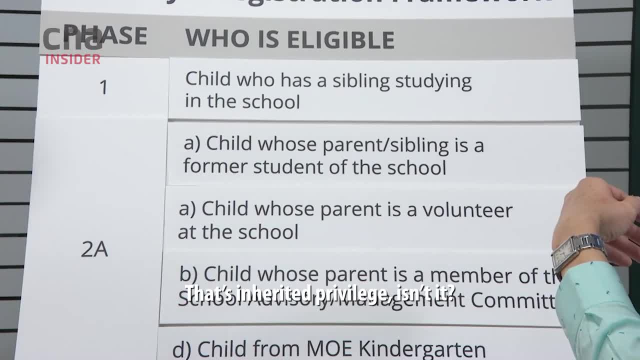 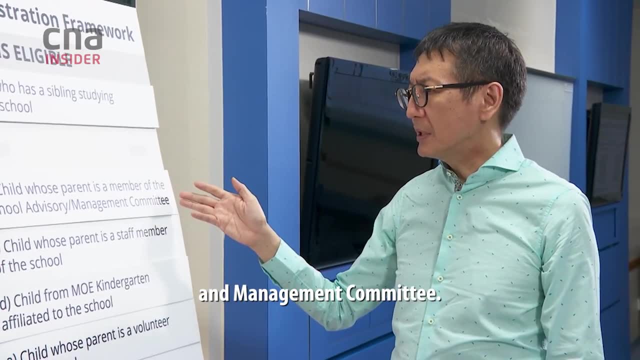 Phase 2A, the alumni. that's inherited privilege, isn't it? Let's take away 2A, 2AA- A parent who's a member of the school advisory and management committee. Once again, it's parental privilege. 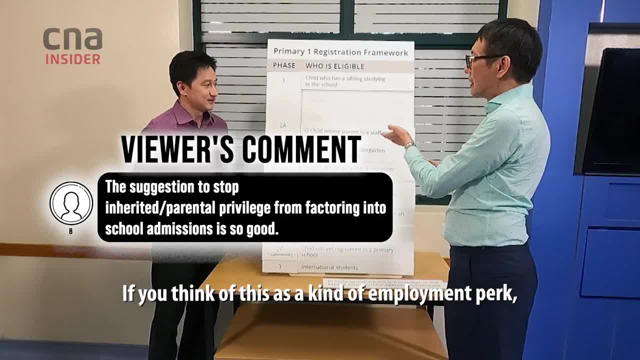 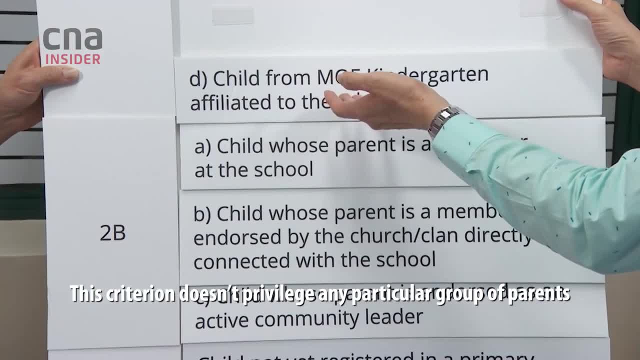 A child whose parent is a staff member of the school. if you think of this as a kind of employment perk, we should say no to this too. Okay, This criterion doesn't privilege any particular group of parents, and we have to remember that these MOE kindergartens. 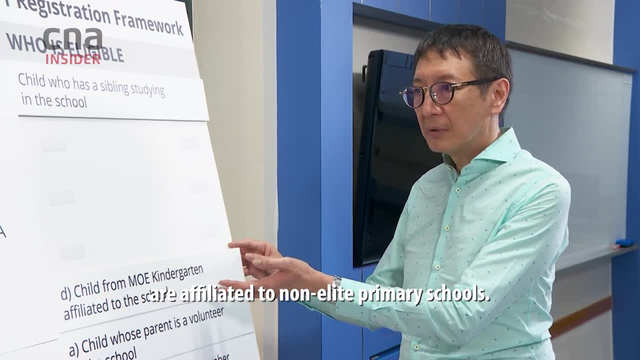 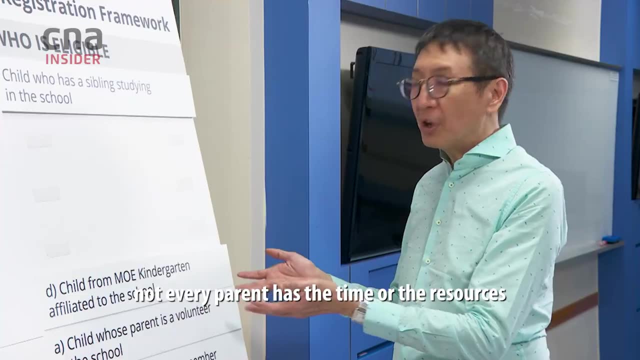 are affiliated to non-elite primary schools. So that's 2A pretty much wiped out. What about 2B, A child whose parent is a volunteer at the school? Not every parent has the time or the resources to be a volunteer. 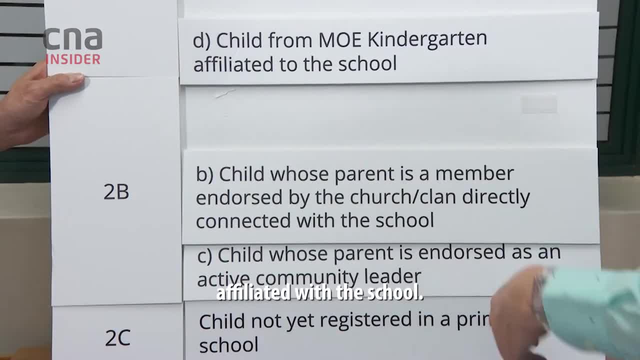 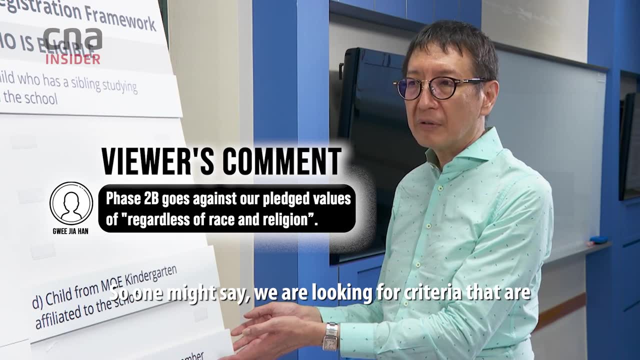 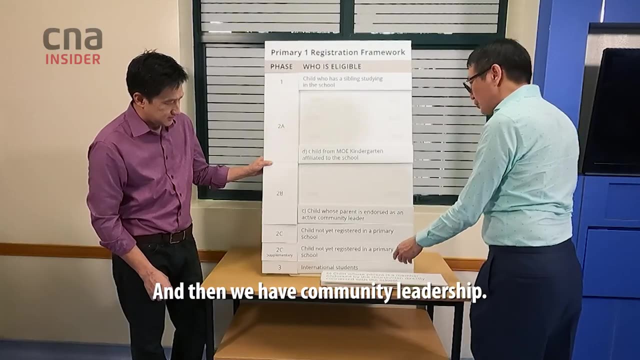 And then membership in a church or clan that's affiliated with the school. This criterion only affects a small minority of schools Right In Singapore. So one might say we're looking for a criteria that are consistent across all of our primary schools, And then we have community leadership. 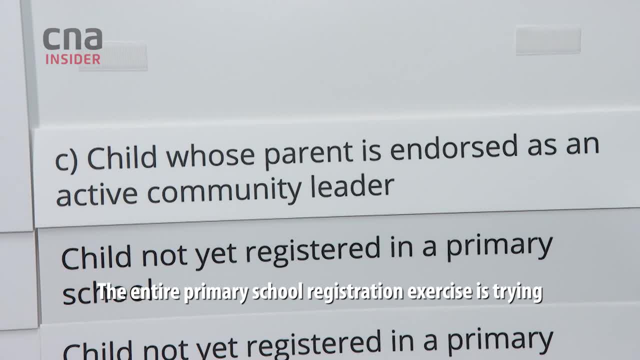 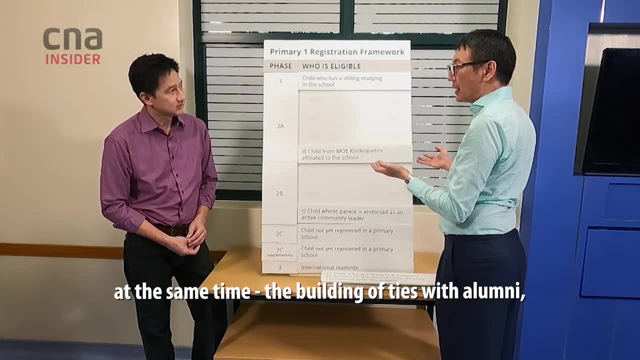 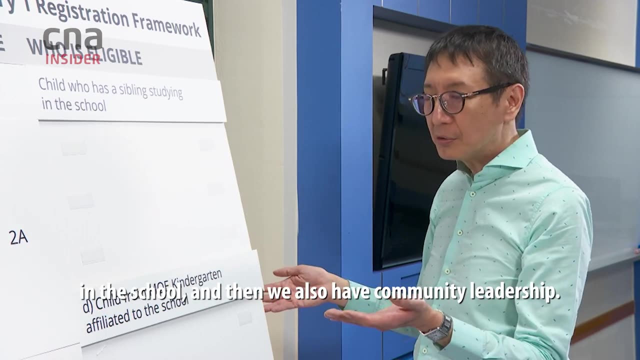 Right. The entire primary school registration exercise is trying to accomplish too many competing objectives at the same time: The building of ties with alumni, the church or clan. employment perks for parents who work in the school, benefits for parents who volunteer in the school. 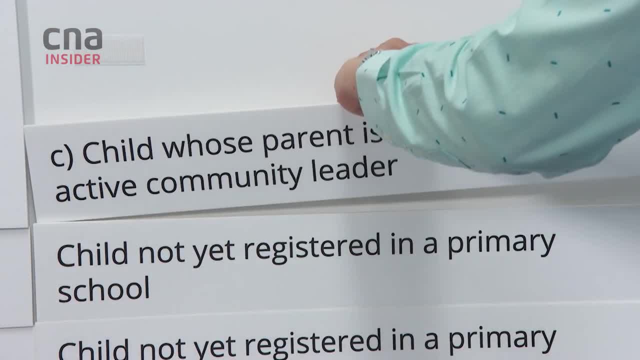 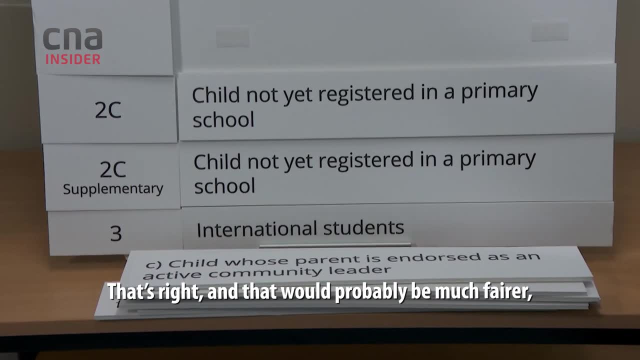 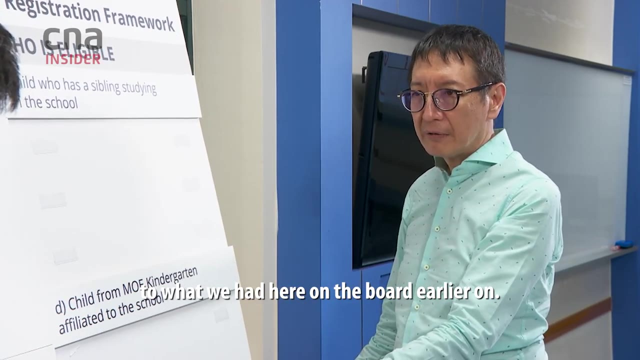 Okay, And then we also have community, Community leadership. So if we look at it, everybody will end up competing at this phase. That's right And that would probably be much fairer in terms of opening up access considerably compared to what we had here on the board earlier on. 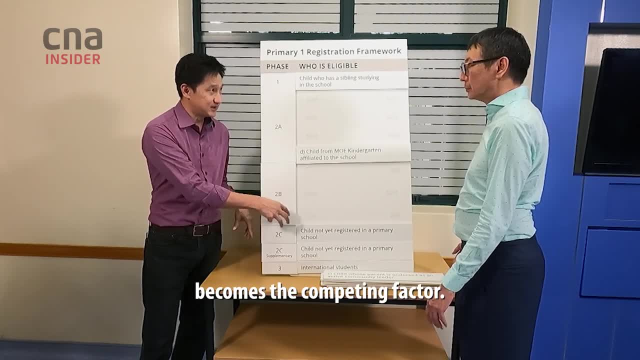 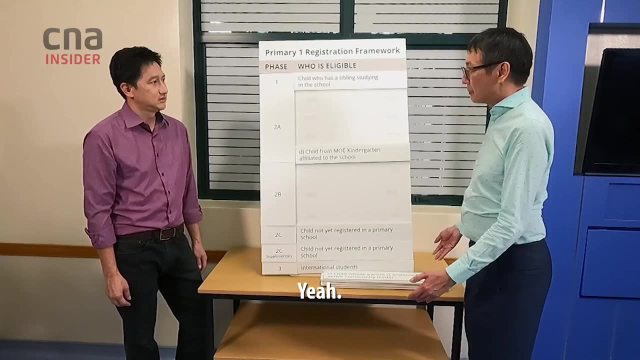 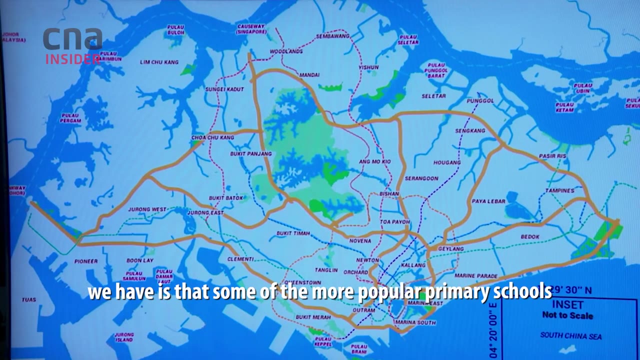 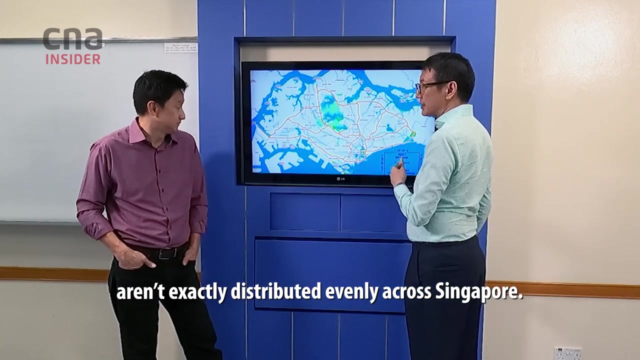 So the one to two kilometre radius of a school becomes the competing factor. I think we need to rethink this whole issue of proximity. Okay, I'll show you. Yeah, I have a map of Singapore here. One of the key issues we have is that some of the more popular primary schools aren't exactly distributed evenly across Singapore. 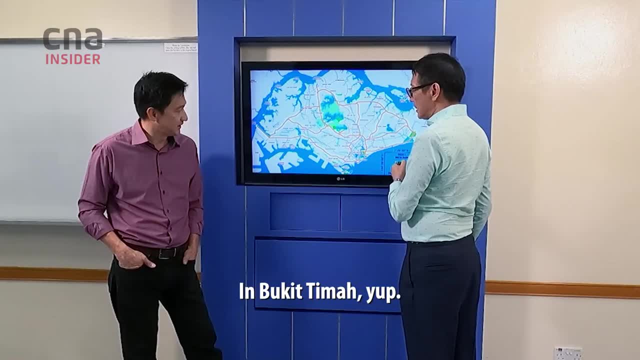 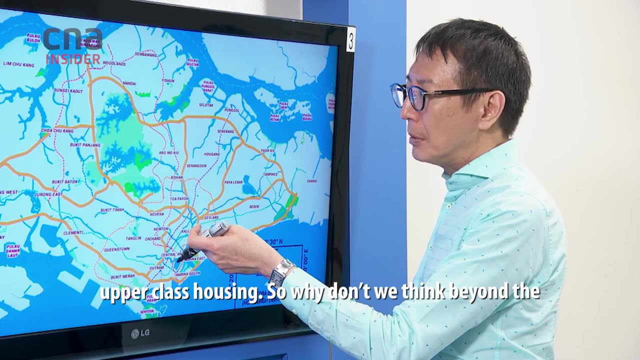 For example, some of the schools in this area here In Bukit Timah. Yeah, That's right, And it's an area that is dominated by upper class housing, Right. So why don't we think beyond the confines of one or two kilometres and say: